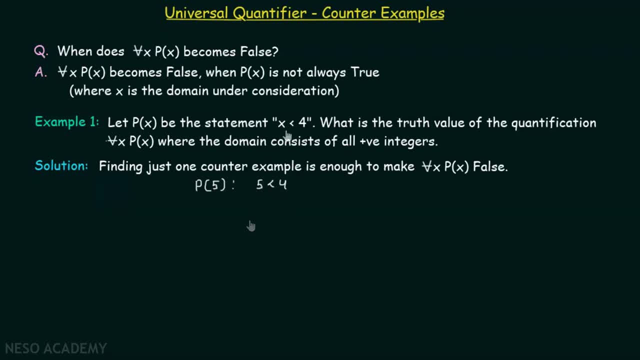 In that case, definitely this becomes 5 less than 4.. We replace this x by 5 and the statement becomes 5 less than 4 and obviously the truth value of the statement is false, As p5 is false. therefore x equal to 5 is one such counter example for the statement. 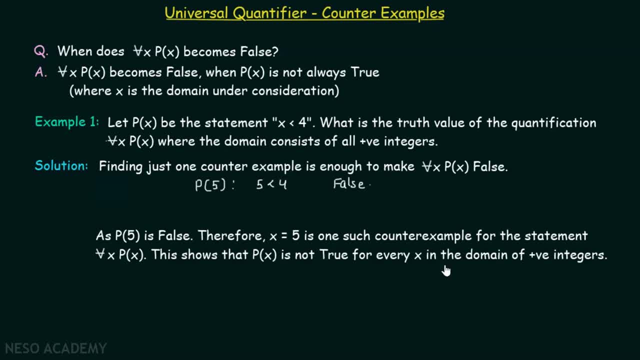 for all x px. This shows that px is false. This shows that px is not true for every x in the domain of positive integers. Isn't that so? This px is not true for every x in the domain of positive integers. Let's consider another example. 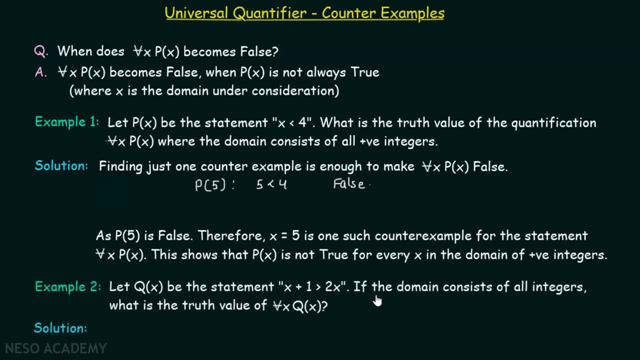 Let qx be the statement x plus 1 greater than 2x. If the domain consists of all integers, then what is the truth value of for all x, qx Here? in this case, we have all integers. We should not only consider positive integers, but we should consider negative integers, as. 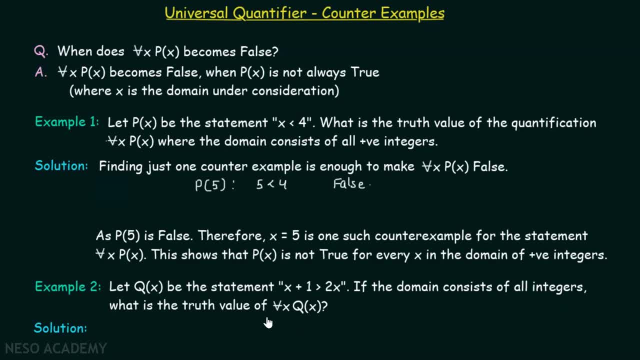 well, Now here, in this case, obviously we need to find out the truth value of for all, x, qx. It could be true, but the better way of finding the truth value is to try to make this false. Just find out one counter example. 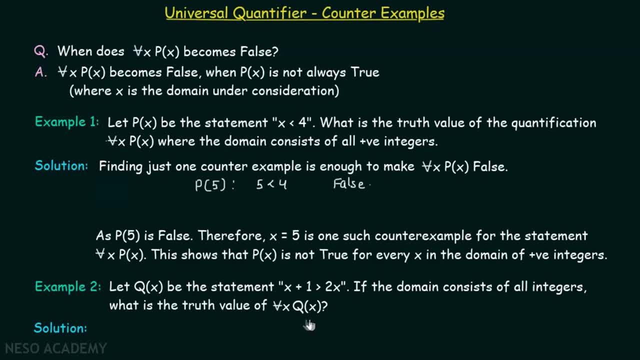 This is much easier, right, Finding the counter example is much easier. So the preferred method is to find out one counter example for which this becomes false, Then definitely the truth value for this will be false. So let's take one counter example. 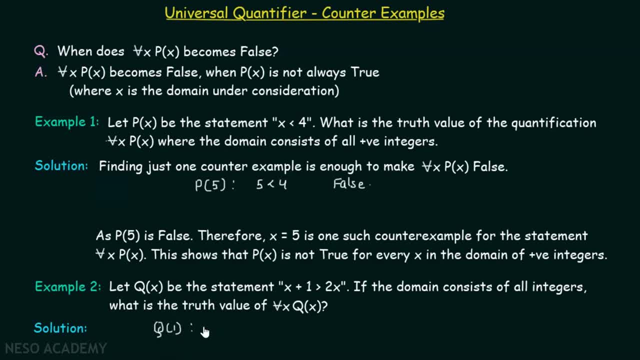 Let's take x equal to 1.. Then in that case, if we replace this x with 1, we get 1.. If we replace this x by 1, then this becomes 1 plus 1 greater than 2 into 1.. 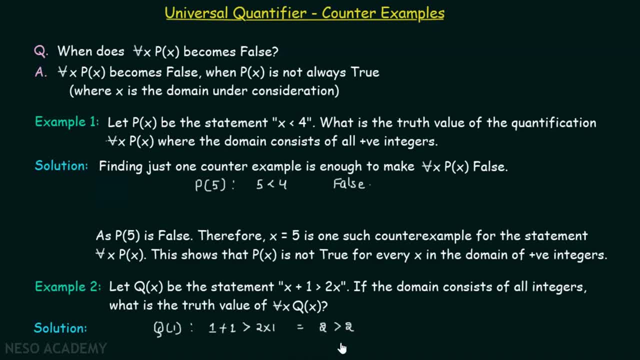 And this is equal to 2 greater than 2.. You know that 2 is not greater than 2.. So we can conclude that, for all, x, qx is false, Isn't that so? So this is the way we can find the counter examples for such statements. 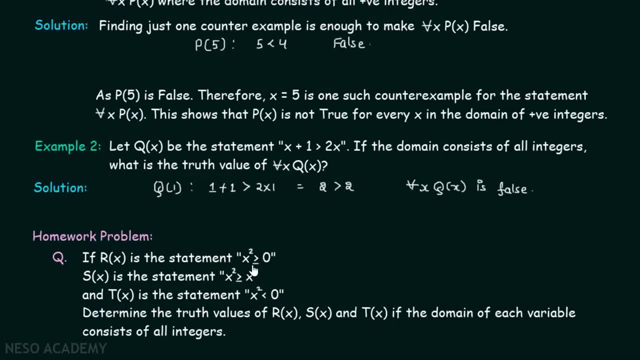 Now here is one homework problem for you. If rx is the statement x square greater than or equal to 0.. If tx is the statement x square greater than or equal to x, Tx is the statement x square less than 0.. You need to determine the truth values of rx, sx and tx. 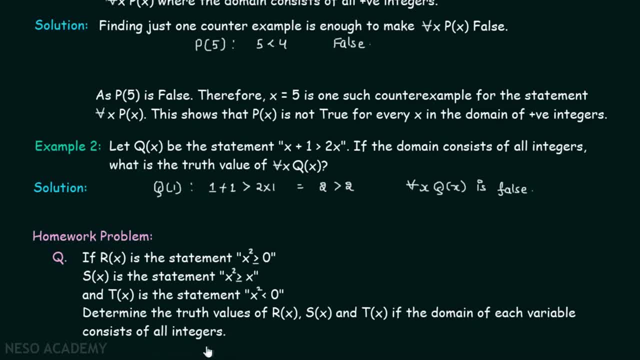 If the domain of each variable consists of all integers. domain is given to you, You need to find out the truth: values of rx- that is this statement, sx- that is this statement, and tx- that is this statement. If the domain is set of all integers. You can always post your answers In the comment section below. 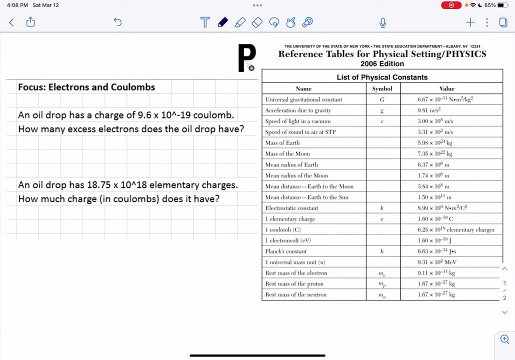 Hi, I'm going to show you how to do the electrons and coulombs do now. In class we talked about elementary charges, which we can find in the reference table right here. Elementary charges use the symbol lowercase e and stand for a value of 1.6 times 10 to the negative. 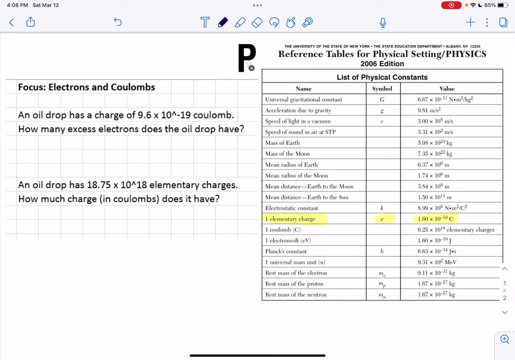 19 coulombs. But when we're talking about elementary charges, what we're talking about is like a single charge. So an electron, for instance, would be an elementary charge. If it's a positive charge, we might also use elementary charges. We usually use these for like small 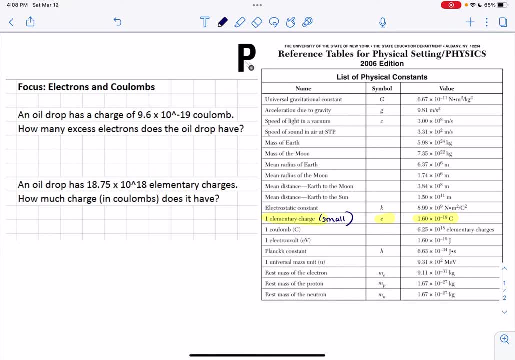 amounts of charge. So if we're talking about a handful of electrons, we're going to use elementary charges. However, later we're going to learn more about electricity and when the electricity is flowing through, like a copper wire, for instance, And in those instances 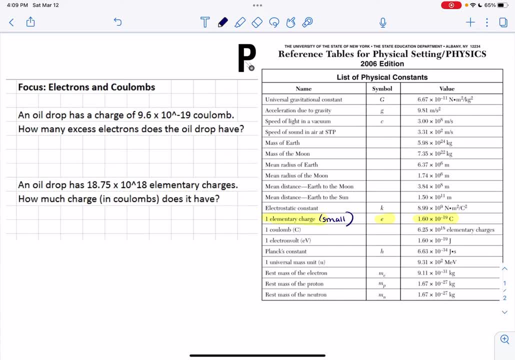 we're going to be talking about a lot of elementary charges. So maybe you're doing the measurements of elementary charges, specifically electrons moving through something. So in that case we aren't going to be measuring in elementary charges, We're going to be measuring in coulombs. So one coulomb, if you notice, is 6.25 times 10 to the. 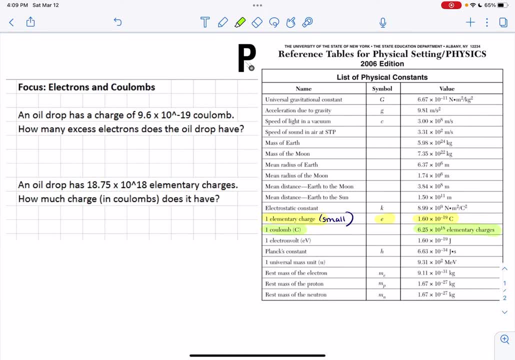 eighteen elementary charges. So this is a really, really big number of elementary charges that make up one coulomb. So one coulomb is often used for a lot of charges that are moving at once peeker, peeking, leak and see, you could kind of get that, but neither am I下來.